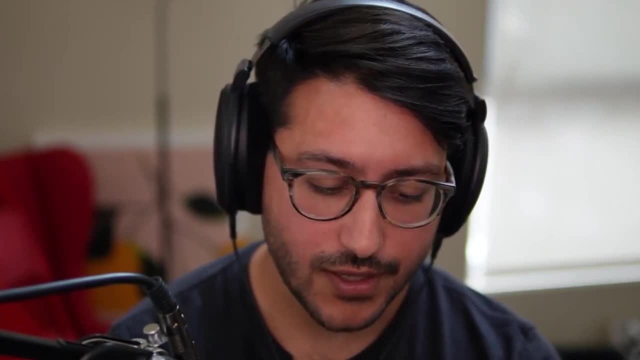 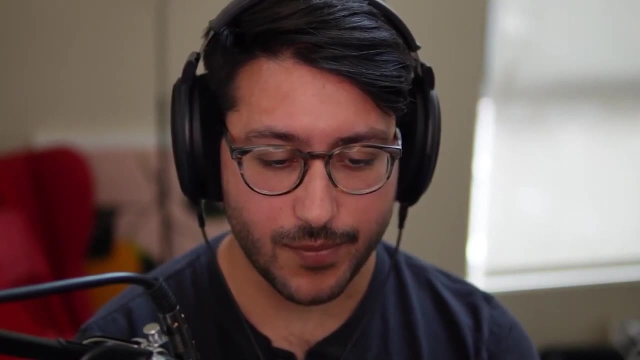 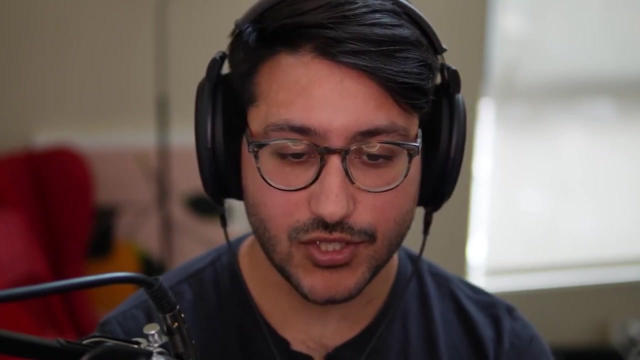 like that, the lingua franca of the data science world, And that makes sense. However, it, number one, raises the barrier to entry for folks who want to be able to create labeling functions that may not know Python, And two, requires, like a fair amount of understanding of the underlying. 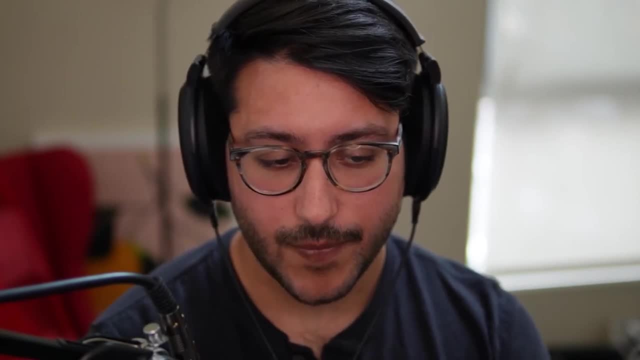 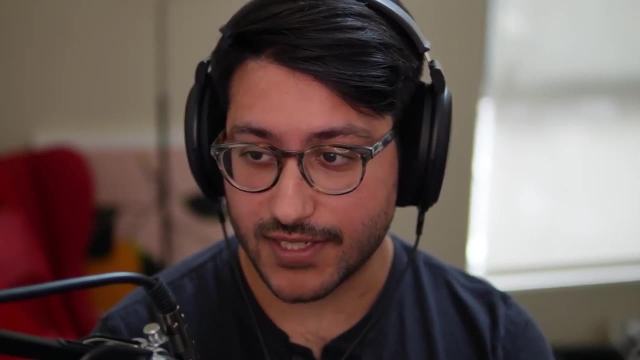 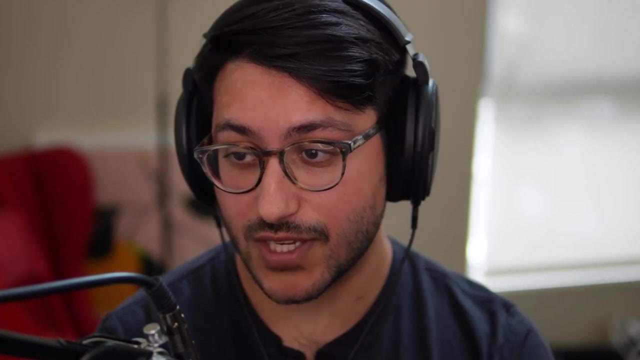 data structure. So, for instance, like you can imagine a labeling function that runs a regex on some text. Great If your input is like a CSV or something. like you can imagine that you're running it over like a particular field or a set of fields or something. But if you 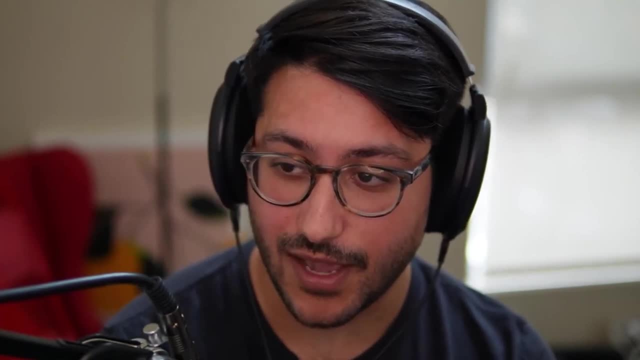 want to like index into some data. if you want to like index into a PDF that's been OCRed and there's like this data structure that you now have to like, interact with. that's like 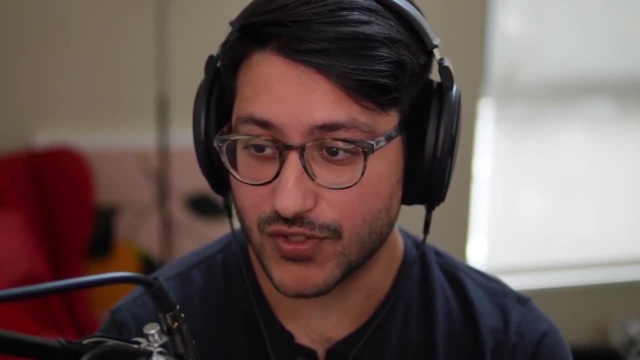 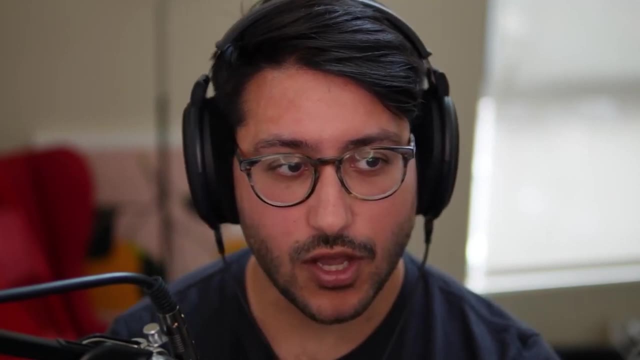 a non-trivial thing for you to wire up when really the thing you're just trying to do is like run a regex, right, Mm-hmm. So that's where, like point number one, Point number two is- we saw an inherent need to automate the process of weak 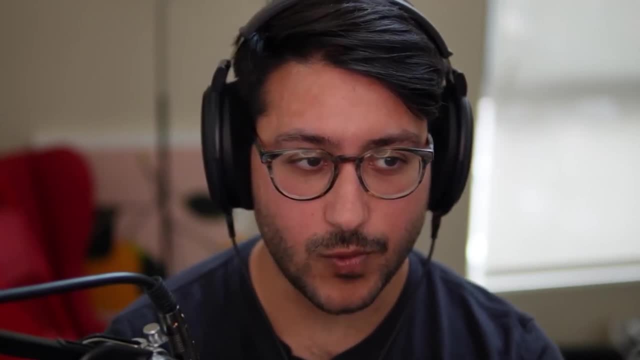 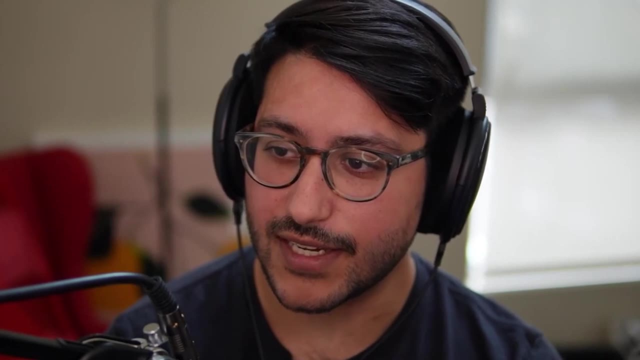 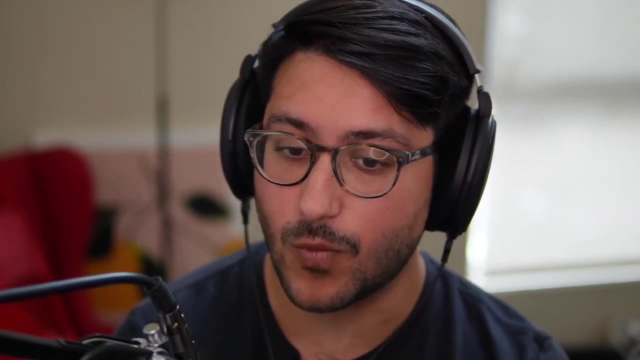 supervision, And what I mean by that is weak supervision at its core. you can think of it as like an ensembling technique. You're creating large quantities of independent sources of signal and you're combining them in ways that produce labels. So really like the weakly supervised. 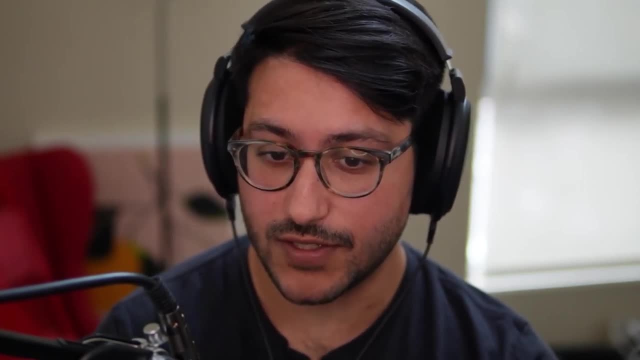 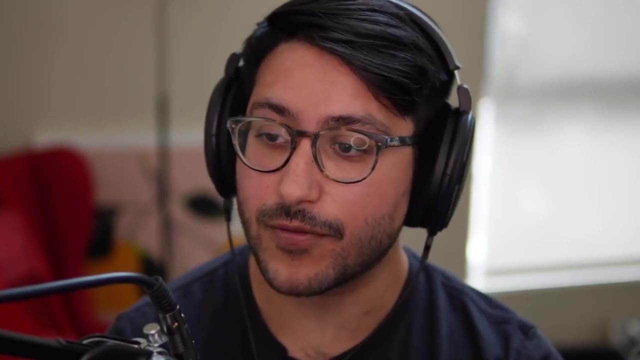 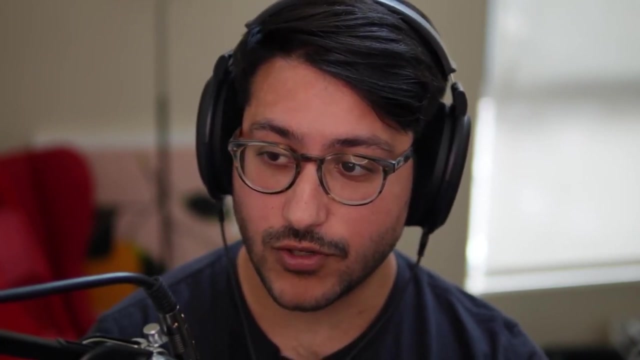 process is just ensembling Mm-hmm, And the question is: what sort of interesting signals can you introduce And like? how independent are they? How many different varieties Like? how much of the problem do they capture? So weakly supervised systems benefit from creating large quantities of these heuristics. 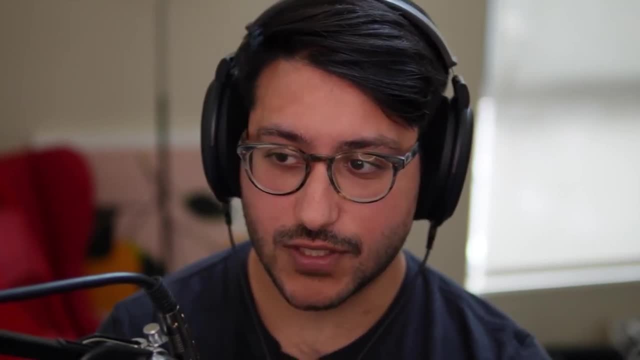 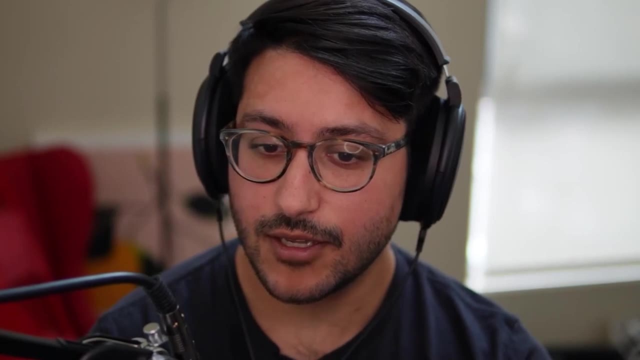 very quickly, And if you're sitting there just coming up with things off the top of your head, it's going to take you a long time. You know, even creating one labeling function will take you several minutes, Mm-hmm, But your problem might be correctly. 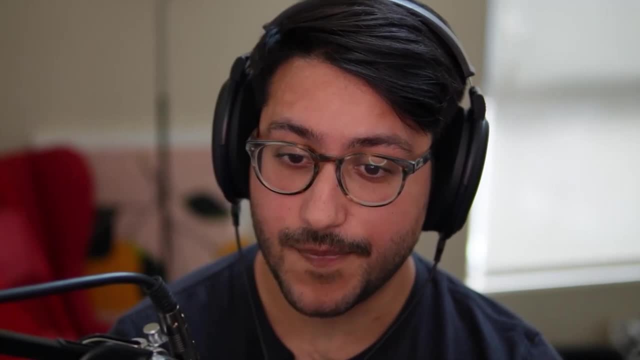 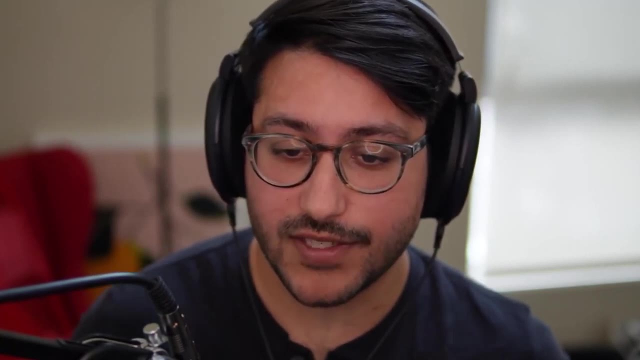 solved with like 200 labeling functions. You don't know ahead of time, Right? So are you going to spend all that time just coming up with stuff off the top of your head? Probably not, So we need ways to generate. 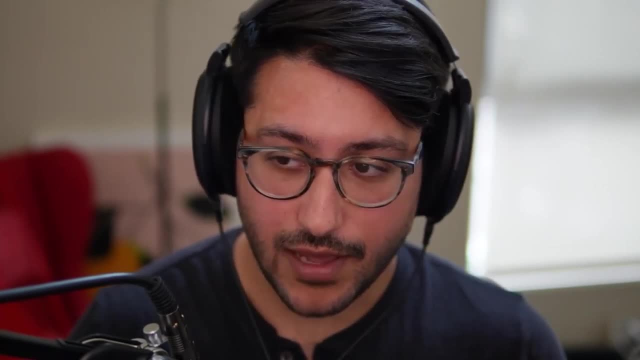 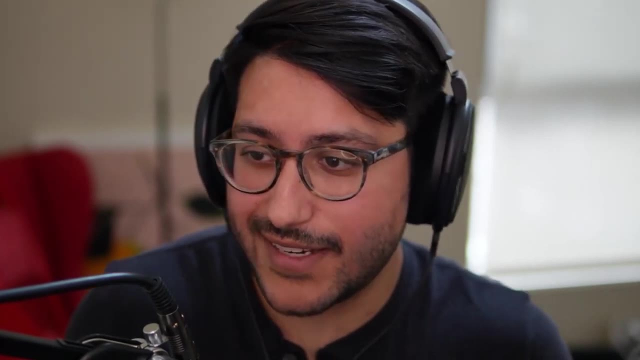 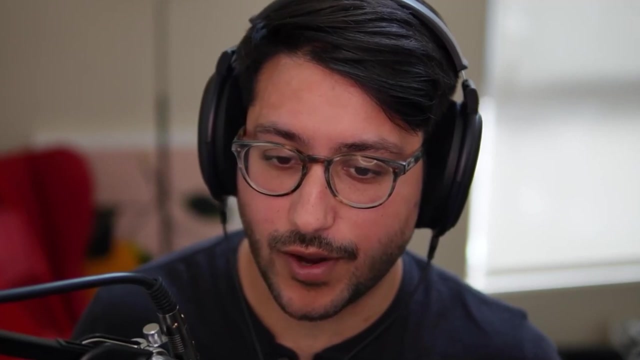 labeling functions, And the problem is Python and pretty much every programming language today can't easily be generated, at least not in a safe way. So this lends itself to like the halting problem, for instance, where in some program you can't predict ahead of time if that program will terminate or not. 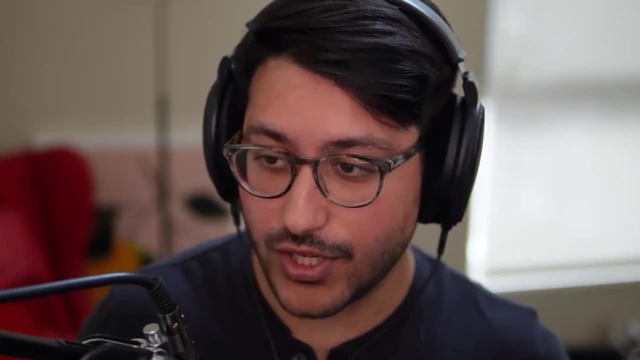 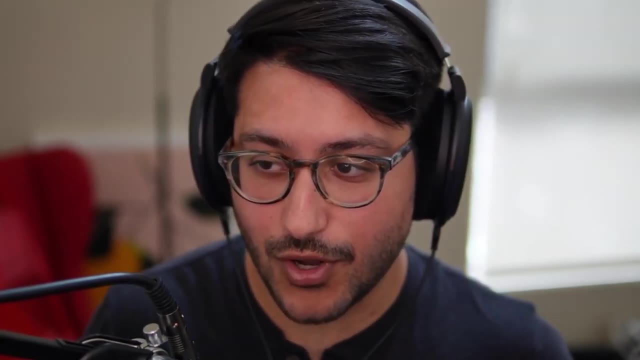 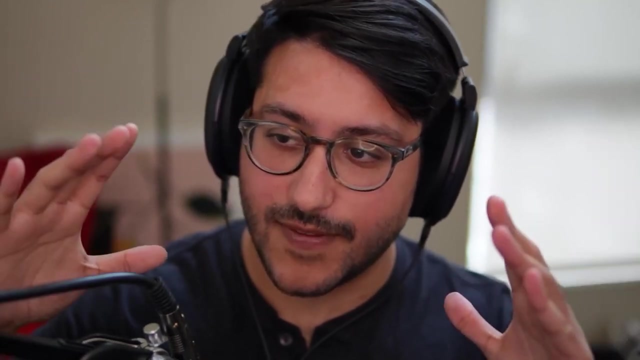 unless, like running it, So like every Turing complete language suffers from this particular problem. So if we were to generate just arbitrary Python, we don't know ahead of time if it's going to be safe to run right. So that means that we have to constrain the space that we're generating. 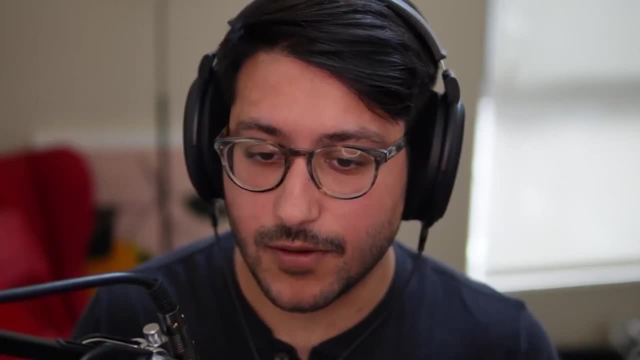 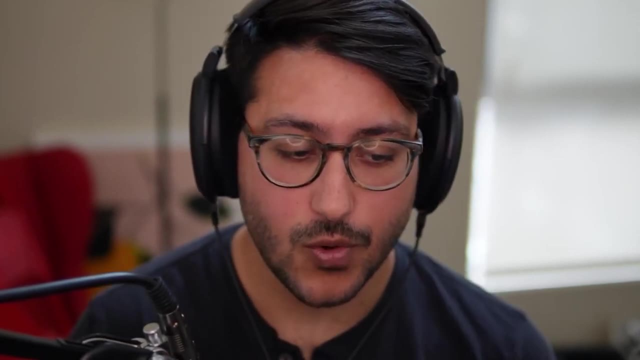 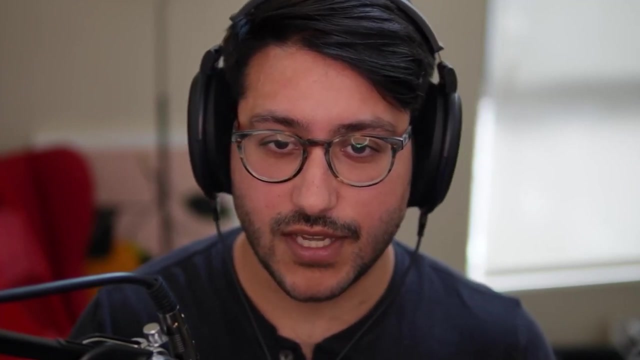 somehow, And that lends itself to a different what's called formal grammar right. And this is like where Noam Chomsky's hierarchy comes in, where you have different types of grammars. So the extremes are, what is it like? infinitely recursive. I forget what it's called. Let me. 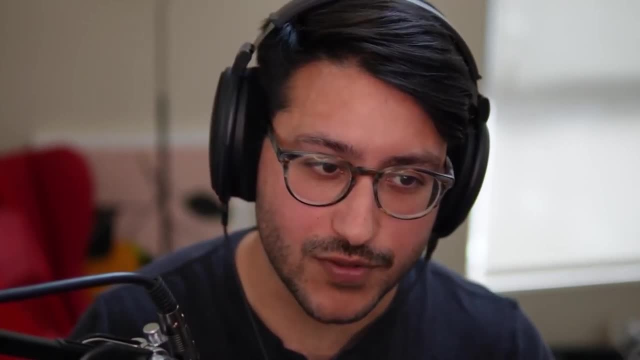 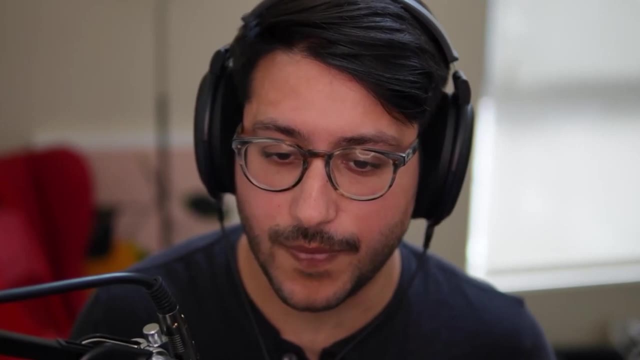 actually quickly Google this Unrestricted grammar. That's what it's called. That's basically like a Turing machine, right? It has like an unlimited amount of context that it can pull from. You have variables that are defined like somewhere else in the program that are: 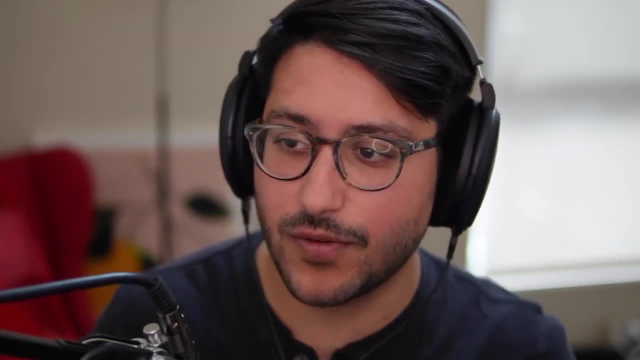 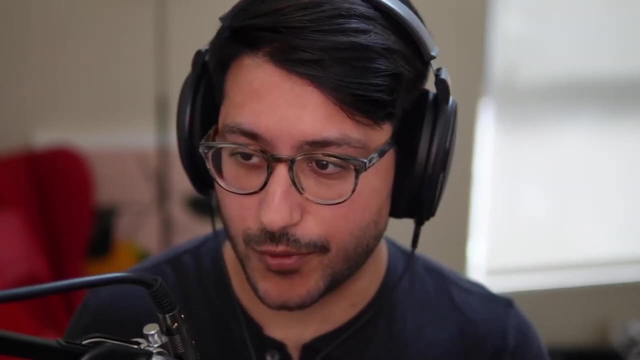 eventually used downstream, Like it requires a lot of context. It requires a lot of context And, again, there's a lot of context to evaluate this thing Versus, at the very bottom layer of the hierarchy, you have what are called regular grammars, which, as an example, you have regular 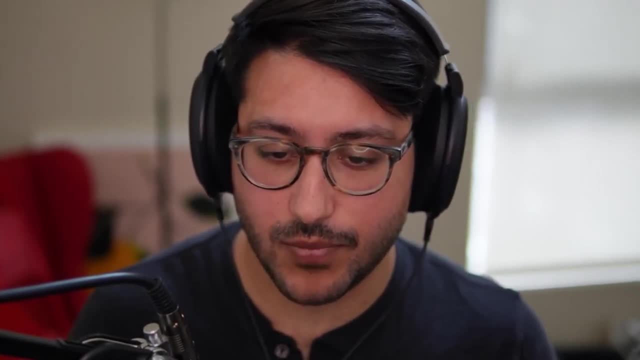 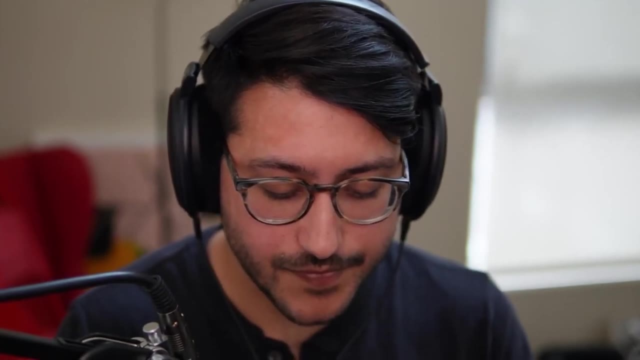 expressions, And these are just things that can be processed by like finite state machines, And the reason why this is important is, if you think about a regex- if I have the regex ABC- all that means is in some text. I want to find ABC And return true to this, And that's why I'm using this. 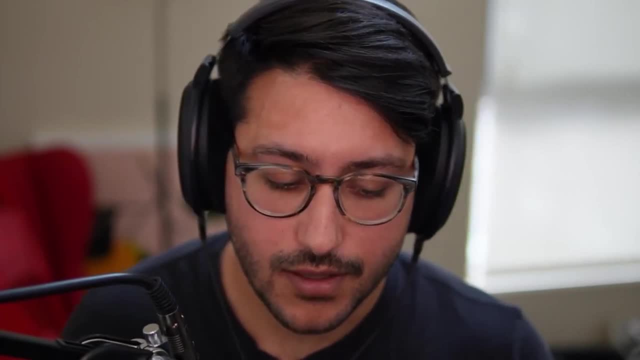 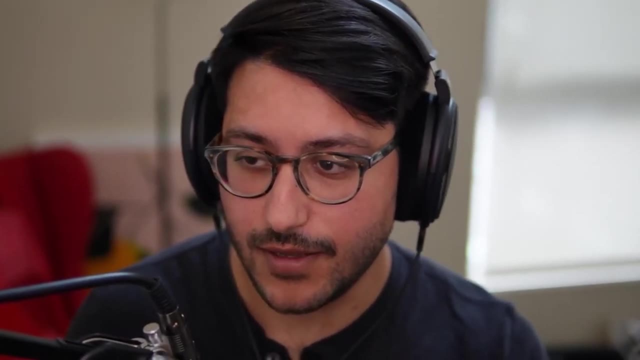 for this particular algorithm. For that reason I'm even using it for other things, And you can use it and return true if I find it. So what I can do is I can actually take the letters ABC and turn it into a finite state machine. I can just say I start if I find the letter A transition to the 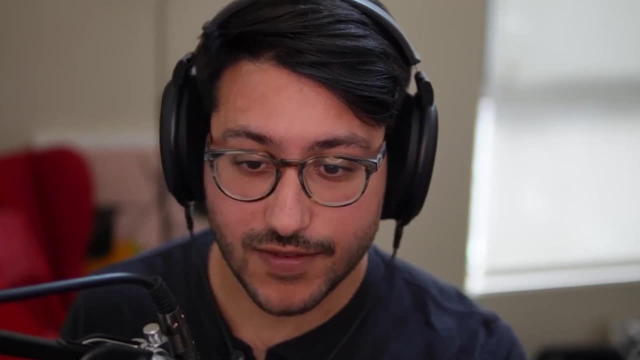 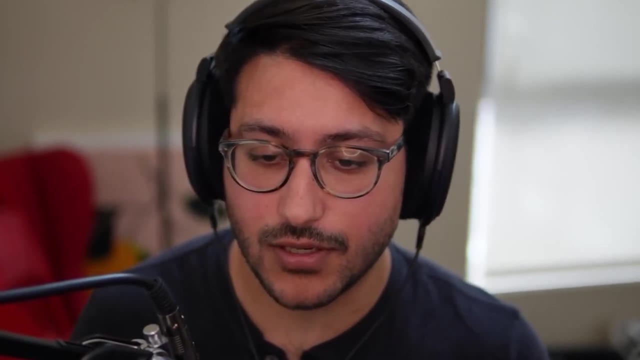 next stage. If I find the letter B right after that, transition to the next state. If I find the letter C right after that, transition to the next state. I didn't need to know anything. I didn't need to retain any information about the previous values that were found or anything that's. 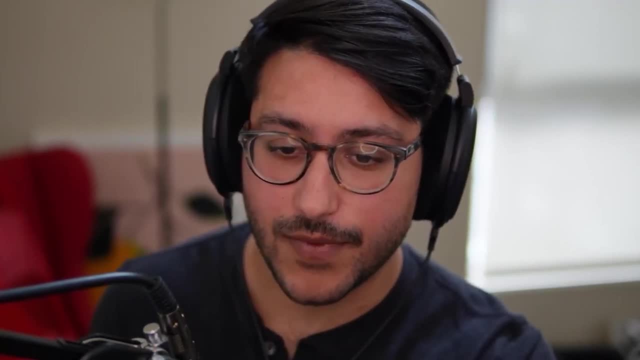 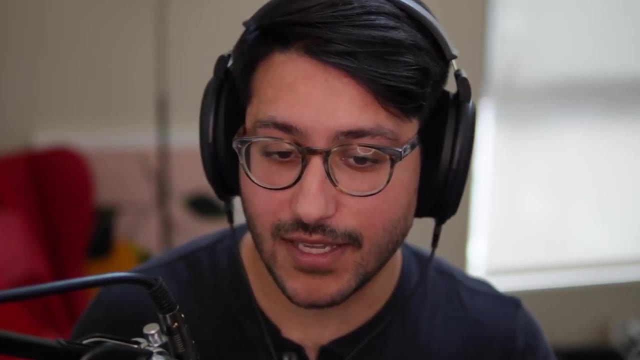 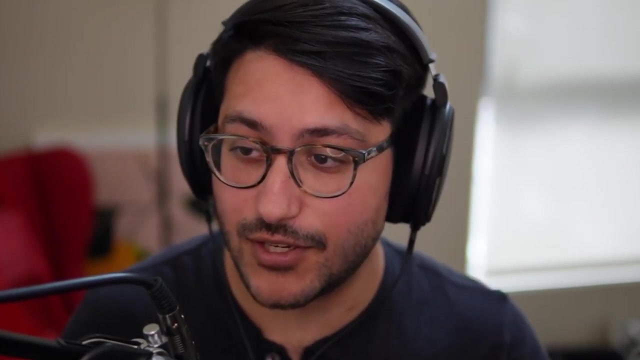 later on. really, I can evaluate this linearly and I can scan through the text from left to right, let's say, and I can process this thing in line, which means that I can efficiently process this and I can calculate if this thing is going to terminate or not. Interesting side note. most regex implementations in Python, Java, that sort of thing are actually non-regular. They don't conform to the regular grammar anymore And that's because people over time have added interesting features like arbitrary forward lookaheads and back references and that sort of thing. That's beside the point. 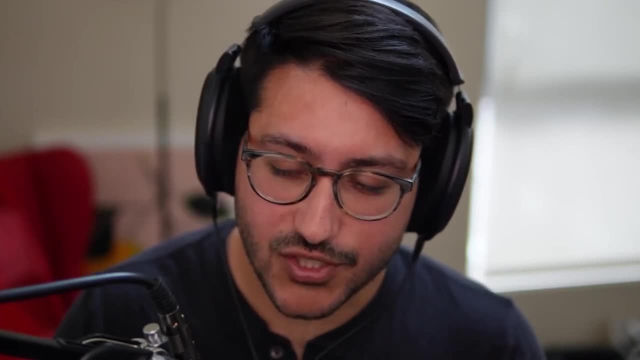 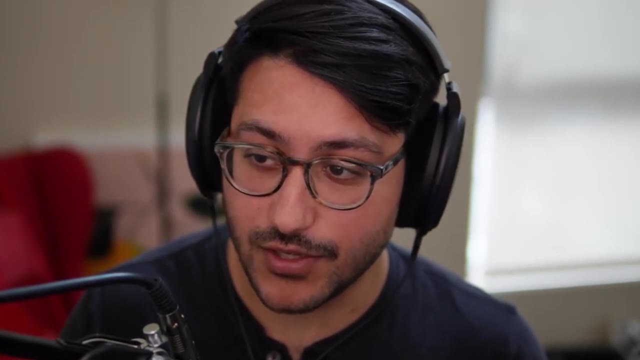 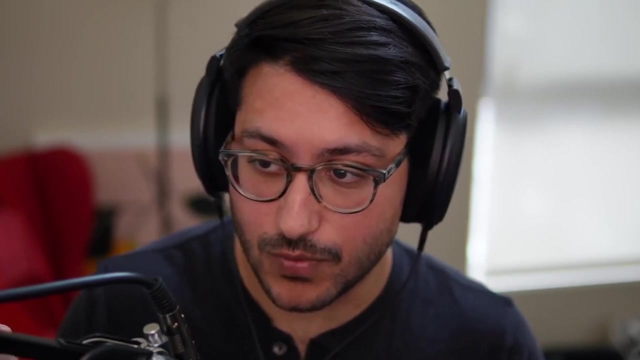 So what we do is we had to constrain the grammar that people were able to use to query data so that we could then simulate it. We could generate it and we know it'll terminate. We know we can evaluate it efficiently, So that implied that we had to basically build a new language Now. 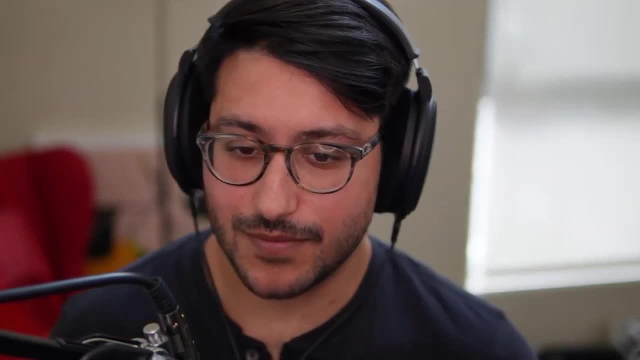 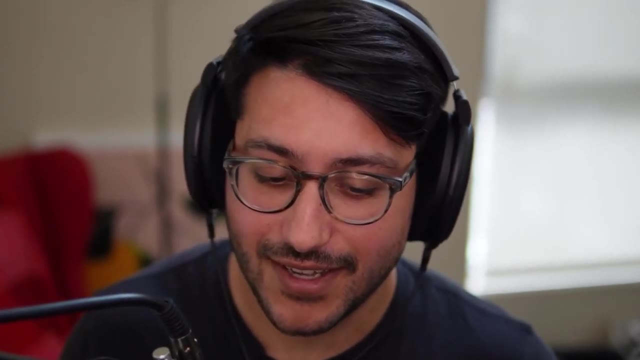 before you design a language, you have to choose like you have to. you have to. you have to choose not to use all the other languages that exist, right. So we had to have very good reason to do that And you know, when we talk about search queries, like there are lots of search, 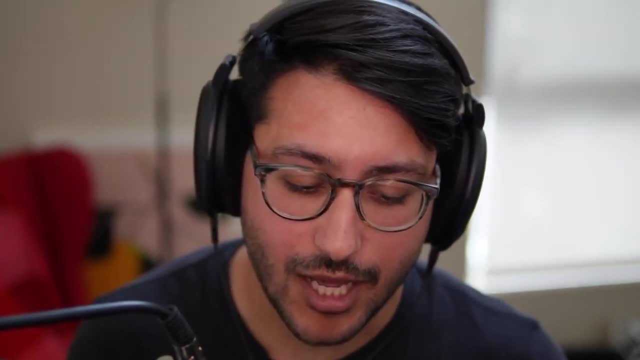 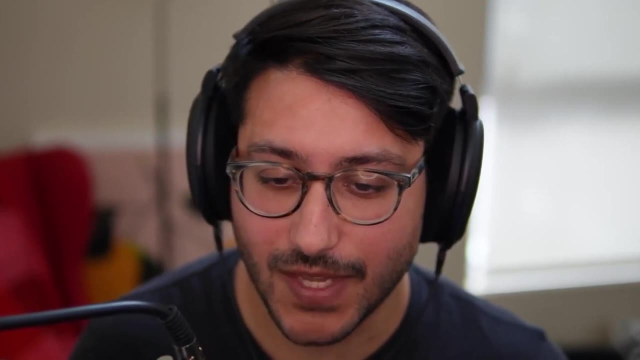 technologies out there that have done exceptional jobs. Elasticsearch is one that immediately comes to mind. So the question that we often get is: like, why not just use Elasticsearch? Like, why did you have to invent your own thing? And the thing that we realize is that 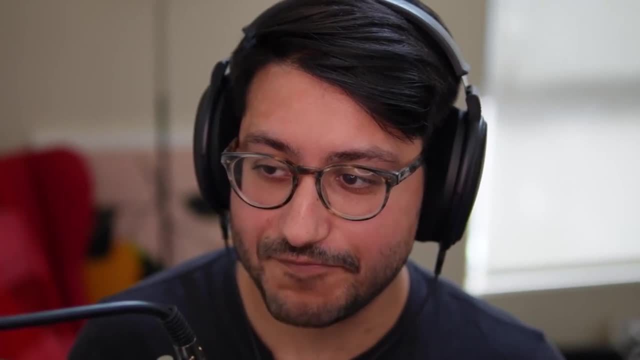 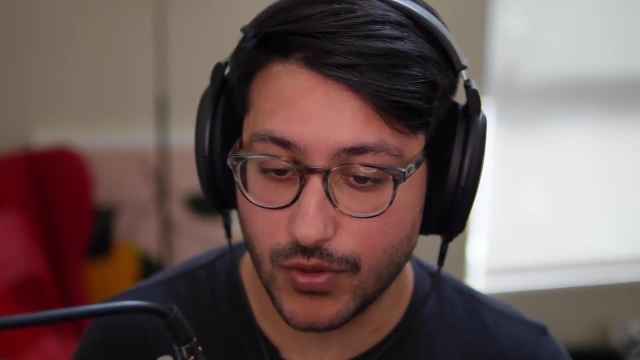 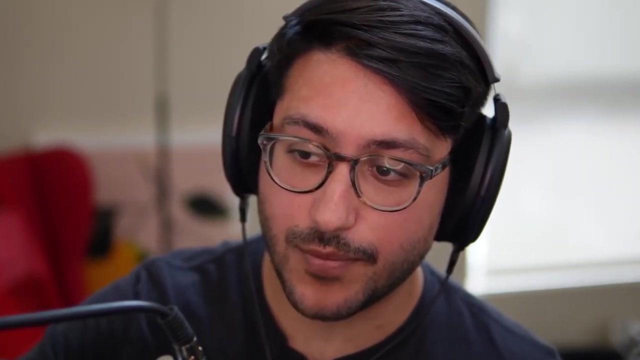 counterintuitively. labeling is a small data problem. You have a finite, fixed data set, typically that you're interacting with. You're usually not labeling in an indefinite way. You typically take a sample from a larger set that you believe is representative, You put it somewhere and you have labelers interact with that And that data. 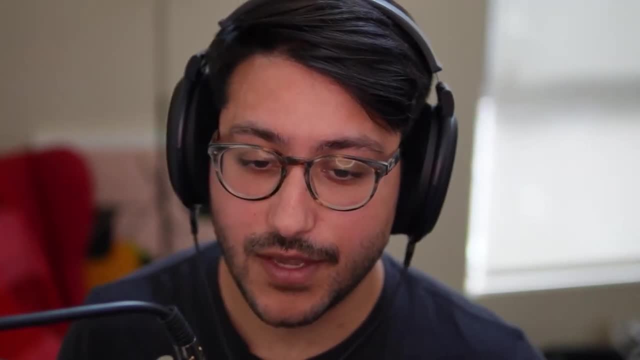 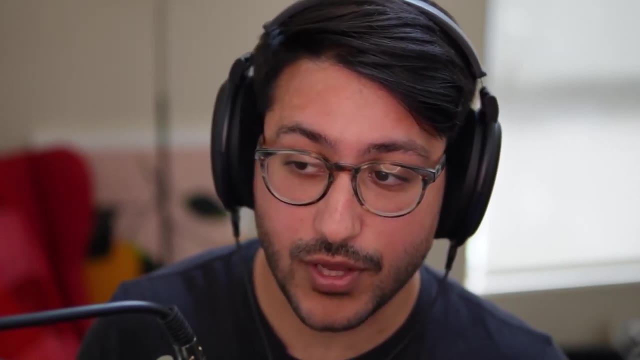 set doesn't change for the duration of that period. So what that means is that Elasticsearch, on the other hand, was actually designed for very large data problems And that data set doesn't change for the duration of that period. So what that means is that Elasticsearch, on the other hand, 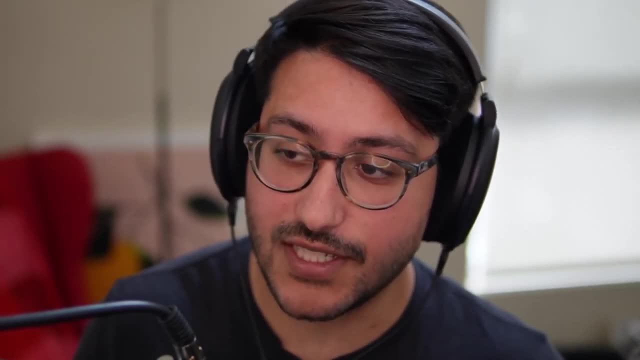 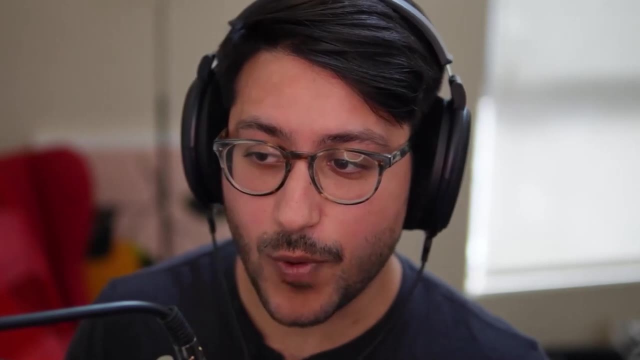 was designed for problems. It was designed for problems where the data actually does need to be split out across many machines and it can't be fit on a single machine, So they've designed clever ways to interact with that sort of data. We don't have that problem, right, And in fact we have the 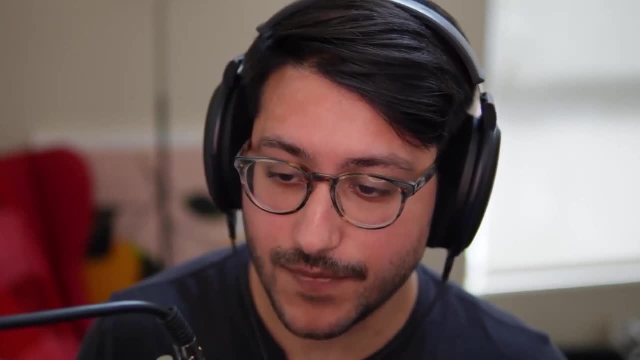 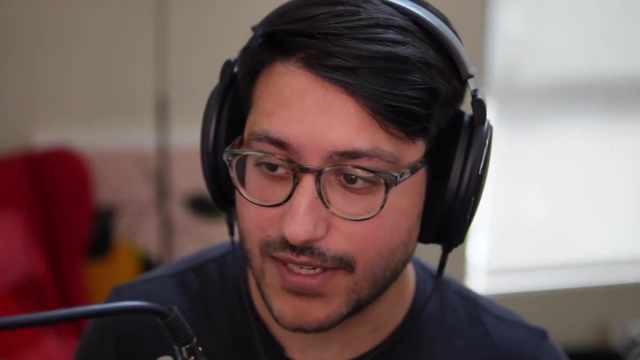 inverse problem. We have data that can fit on a single machine or parts of data that can be fit on individual machines. let's say, And we want to interact with that data as quickly as we possibly can, again to stay in that flow state. How do we do that? So things like Elasticsearch didn't. 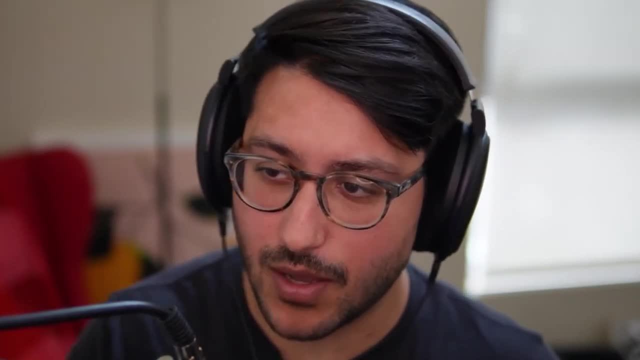 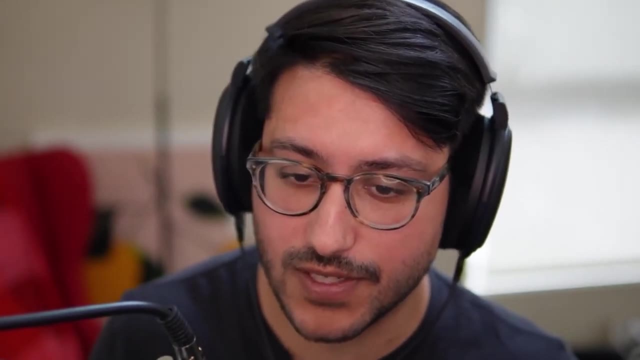 quite work And, not to mention, the language itself became cumbersome for the types of things that you'd want to do from a labeling perspective. You don't just want to be able to do things like keyword searches, You want to be able to do things like similarity searches, like how close is this? 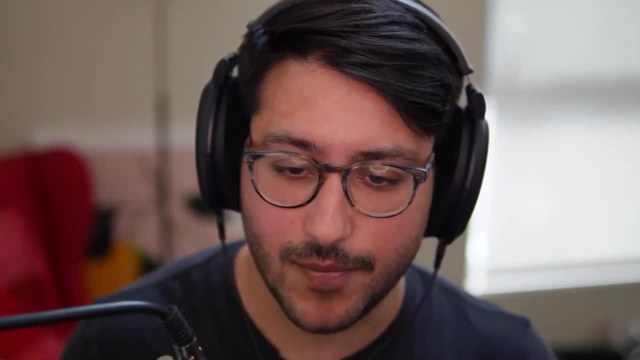 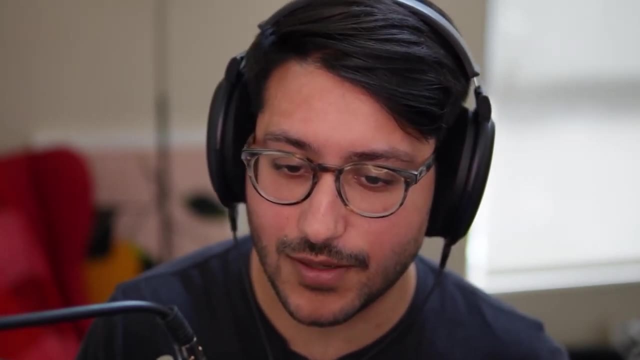 thing to this other thing. You want to be able to do things like database lookups, like all sorts of stuff. So we had to create our own language, which then implies that we had to create our own query engine, the thing to process the language and turn it into something that we can evaluate. 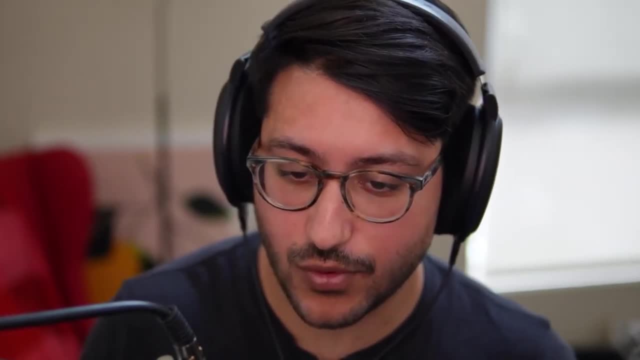 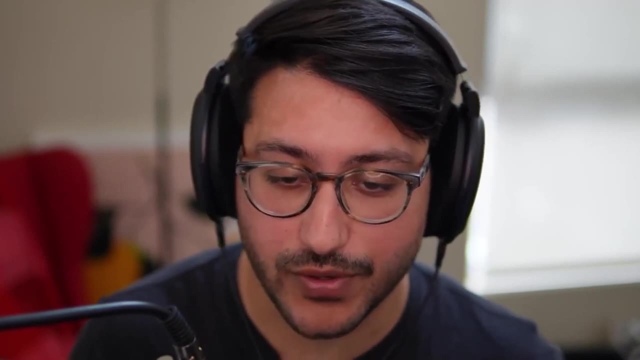 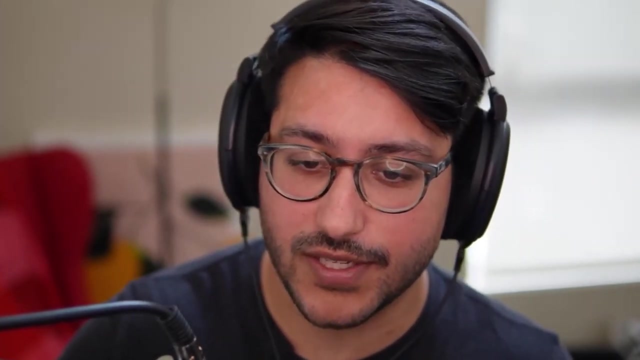 which then also implies that there is a data structure that we've created that allows you to efficiently index in the ways that you'd want. So, whether you're doing full-text classification, whether you're doing NER, like a segmentation-type problem, even into images, video, audio, et cetera, we believe that all these problems share the same. 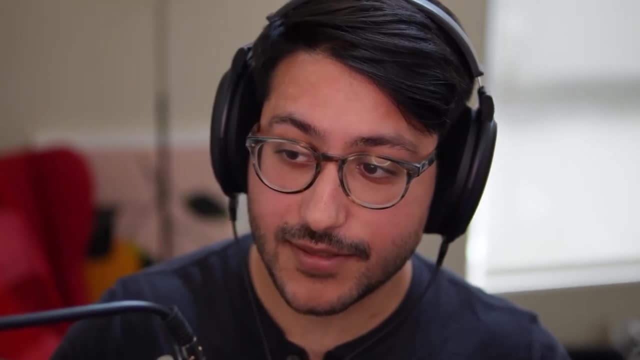 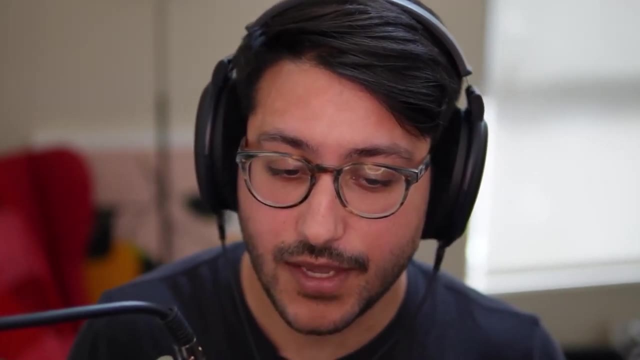 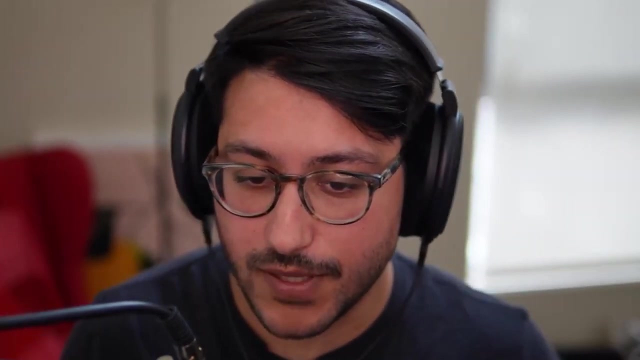 relative footprint, where I have bytes that are laid out in some way that makes sense to the machine and to the users. but I have bytes fundamentally And I have a graph that points into those bytes. So the nodes in the graph could be things like: 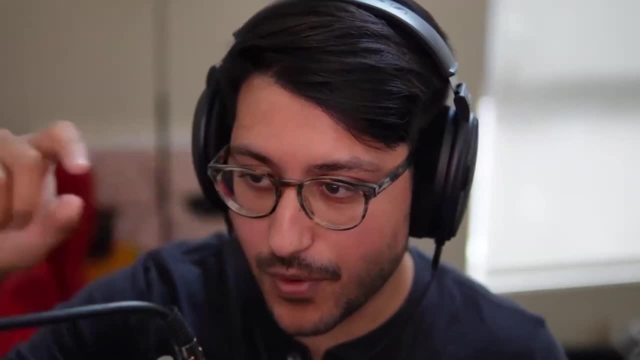 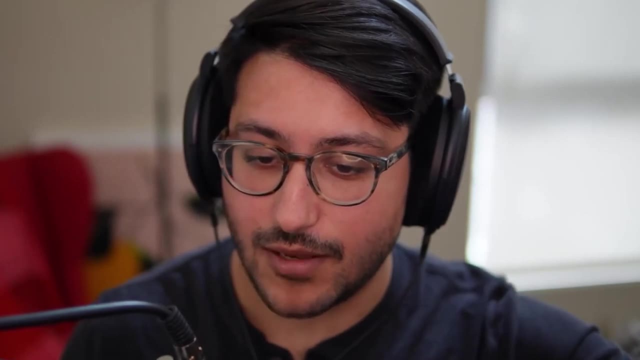 hand labels that people have created and said, okay, this part of the text is such and such label. It could be these labeling functions that are pointing into the data and be like: these are the parts of the data that I affect. It could be what we call derived labels. 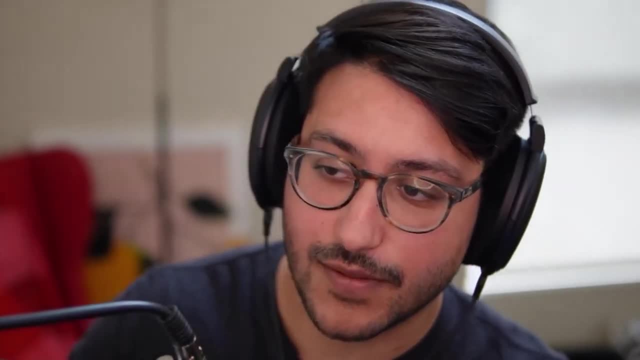 things like labels that are predicted so probabilistic labels that we generate from the contents of our data. We could be able to do that in a way that allows us to do that combination of all your different heuristics. Fundamentally, these are all just nodes in. 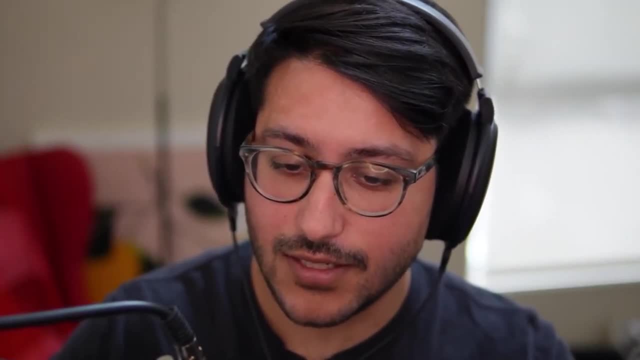 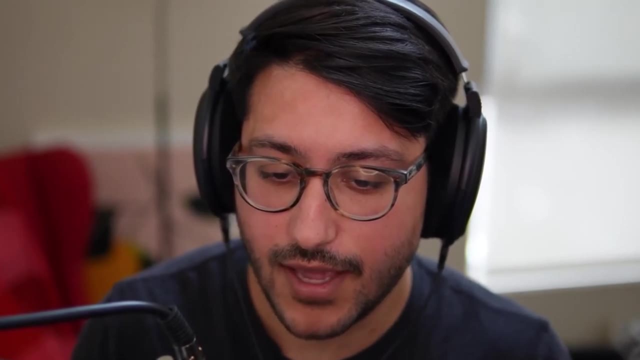 a graph that are pointing into data, And to access that data, you could either access the data directly or you could go through the nodes and say: show me everything that has a greater than 90% likelihood of being such and such class, Or show me everything. 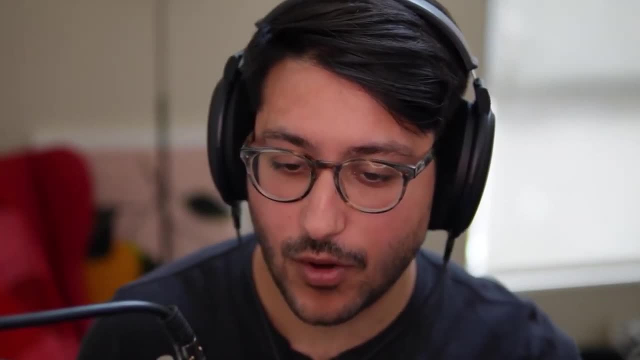 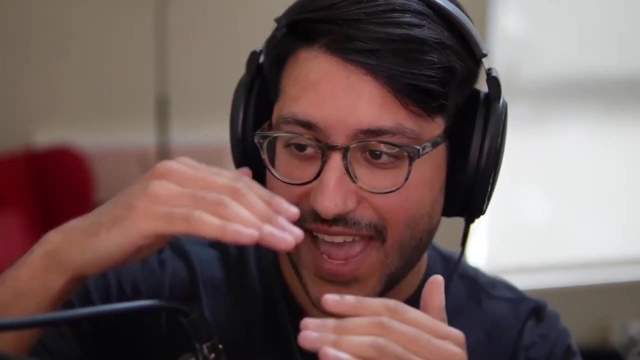 that this person has hand labeled over this period of time. All of that is just metadata stored in a graph that indexes into this data, So we have this like stack of things we had to build in order to do the really cool thing which we're really excited about, which.